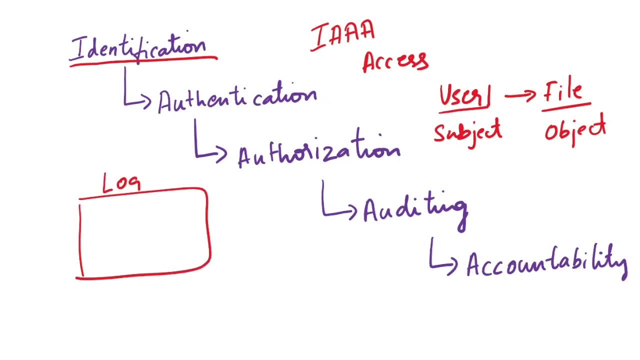 access a web application on a portal, it usually asks you to log in. When you provide your username on that login page, like, for example, your user ID, your email ID, account number, all those are identifications And if it is an application or process, it can be a process ID application ID. 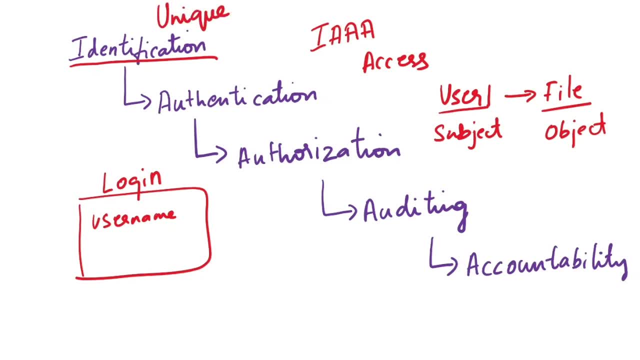 okay, And most of the times the identity is is unique, except for, like, admin users, right? You just have a user ID called admin. That is not unique And most of the times the subject's identity- right, It is public information, Like. 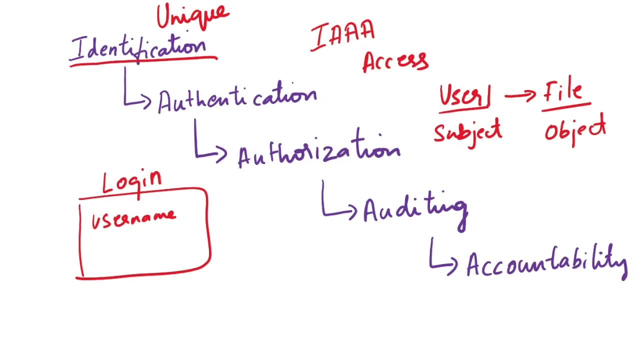 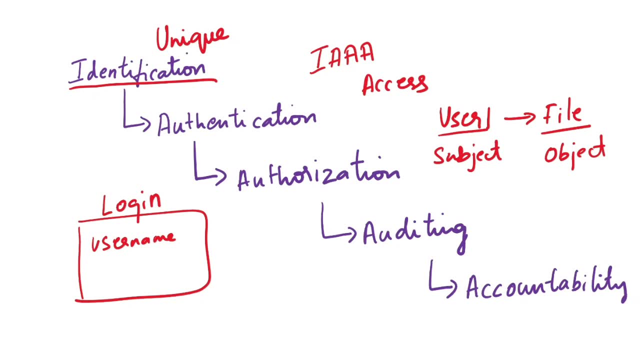 for example, your email address, your name. everything is public, Everybody knows about it. So you cannot log into an application just by having your identification, Like, for example, your username. you'll also have to verify it. That verification step is called as the. 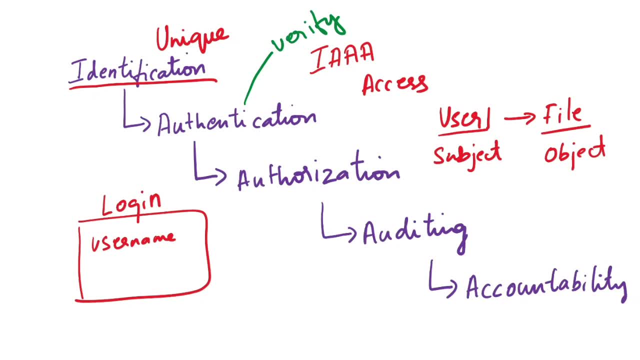 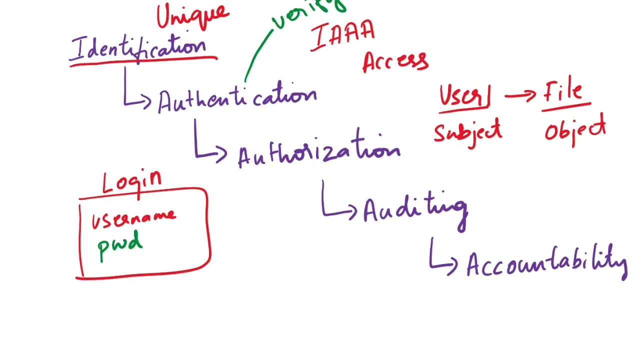 authentication, That is, you're verifying the identity that you claim to be in a simple web application. How do you verify it? by providing your password. It can be passphrase, password, anything, or you know, it can be your pin. So the first step is identification and access control, And the 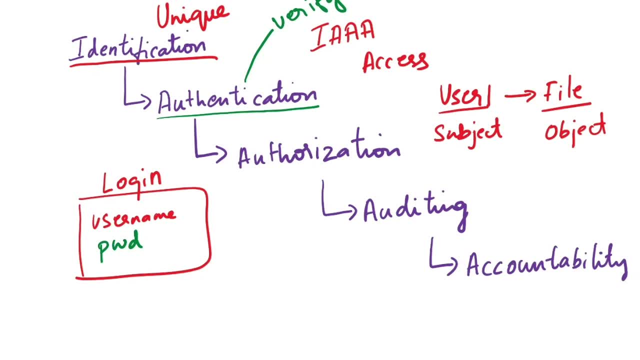 next step is authentication. That is nothing but verifying the identification. So the username is public information, usually, and the password is private. The subject knows what is the password, right? So there are many different types of authentication. Let's see what are those as well. Type one authentication is something that you know. 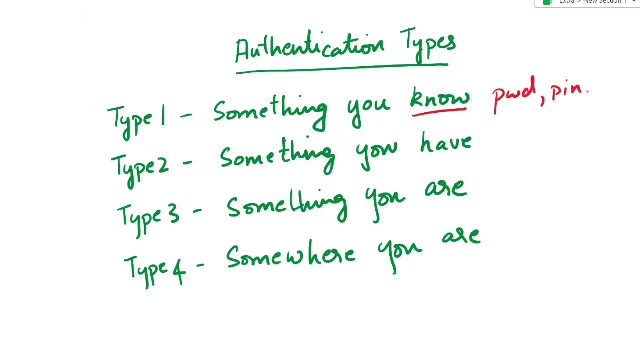 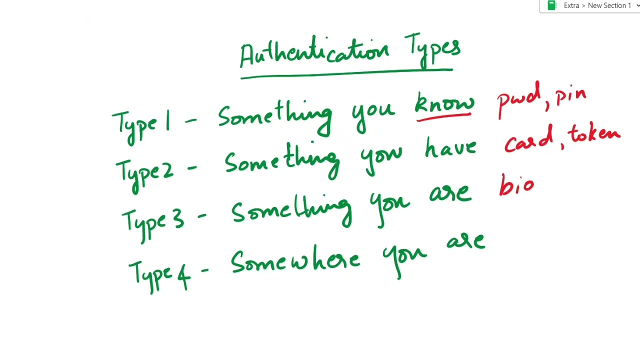 like, for example, your password. there is a pin number that you know or a passphrase. Then you have type two, something that you have. it can be like an access card. it can be a token. Type three is biometrics. okay, That is, your fingerprints, your retina scans, iris scans. 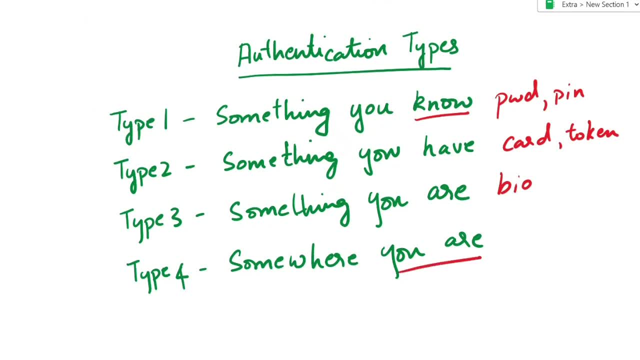 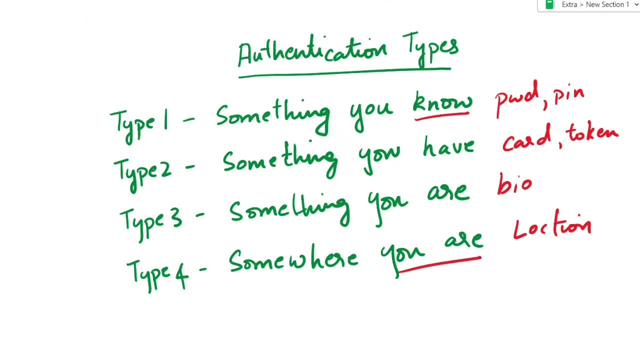 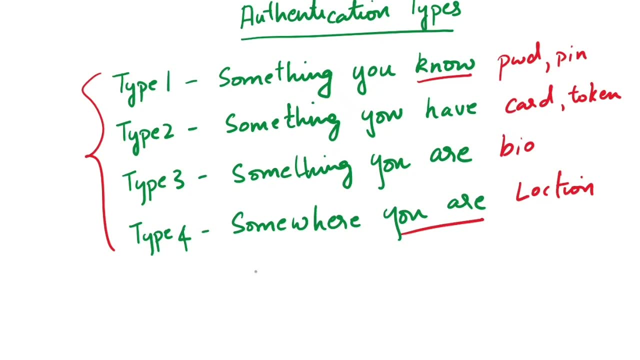 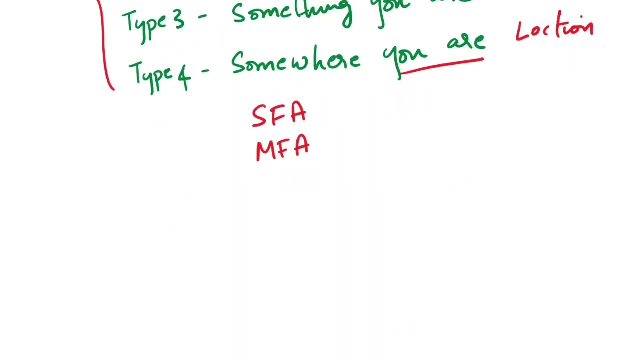 only provide access to an application only if you are in the office network. So these are the types of authentication. Then we also have something called as single factor authentication, SFA, and multi-factor authentication. Single factor: it is the simplest form of 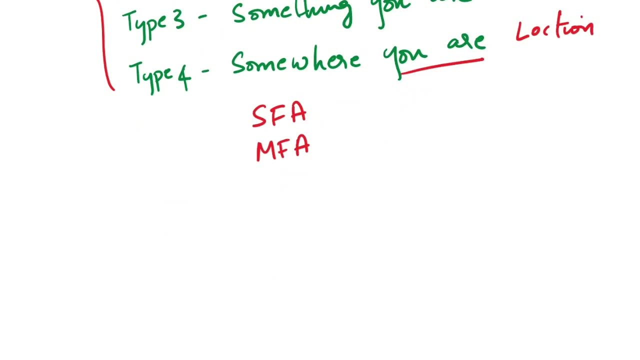 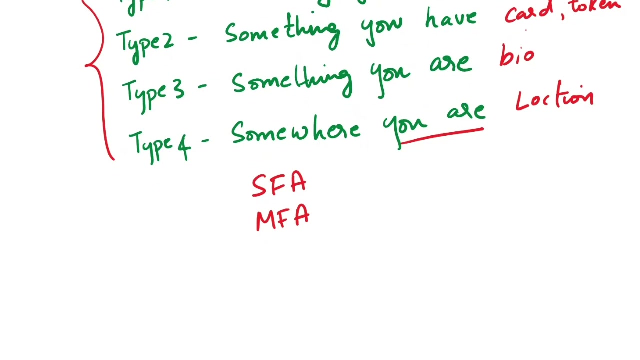 authentication like, for example, a user, an application or a process or a device will have to provide only one type of authentication, like maybe a password or a card, biometrics or just the location. That's it okay. And then we have multi-factor authentication, Like the name. 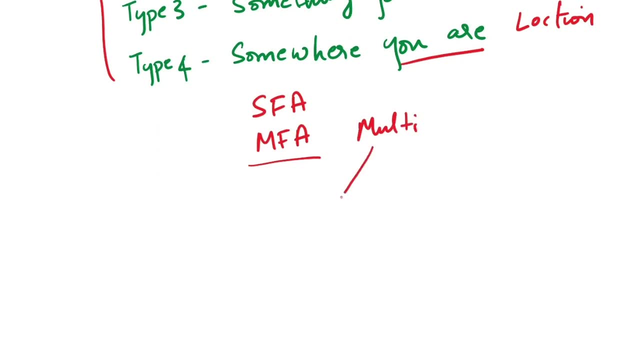 suggests you are using two or more factors, Like, for example, you're using a password as well as a token to log in, And then you have multi-factor authentication, like, for example, you're using a. It is considered to be the strongest form of authentication. So something to remember is that 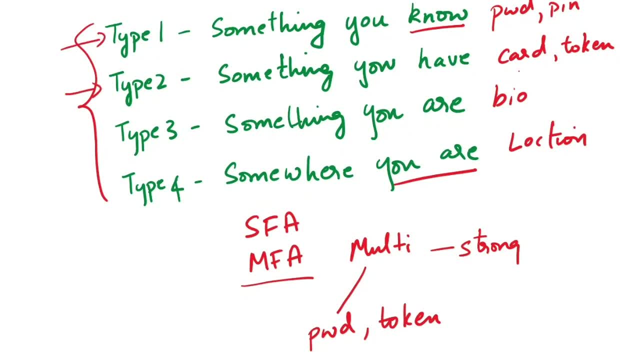 you'll have to use two types for multi-factor authentication: type 1, type 3, or type 2, type 4, or type 4, type 1.. You cannot use password as well as PIN from type 1 and say that is. 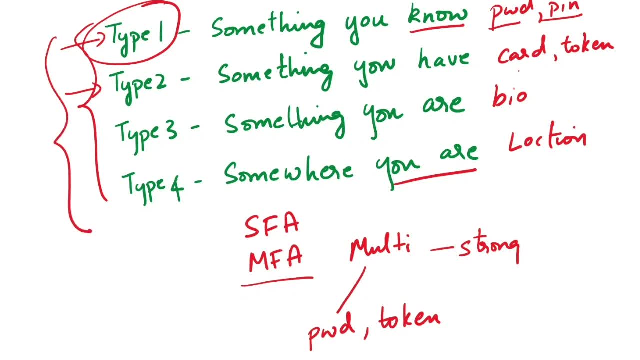 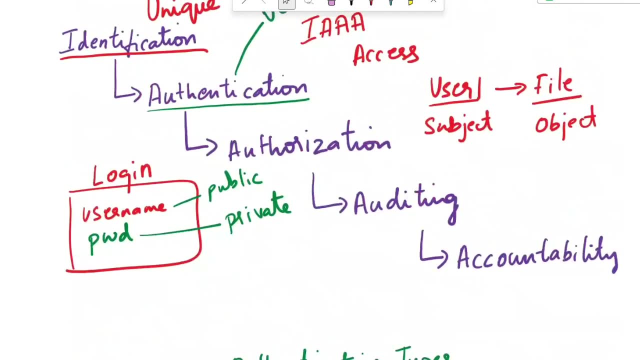 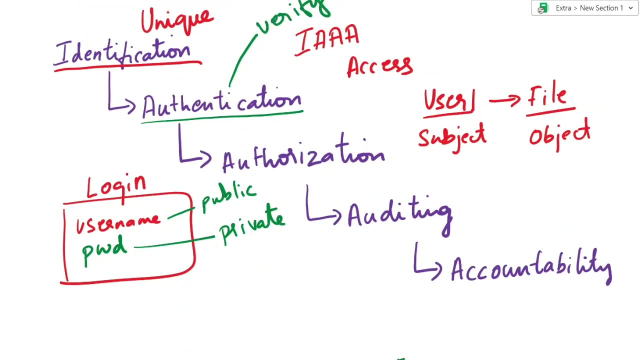 multi-factor authentication. It should be from different types, and only then it becomes multi-factor authentication. okay, Okay, now going back to identification and authentication. first step is identifying the subject, second step is verifying the subject and then comes the authorization. Once a user is authentication, the access must be authorized. 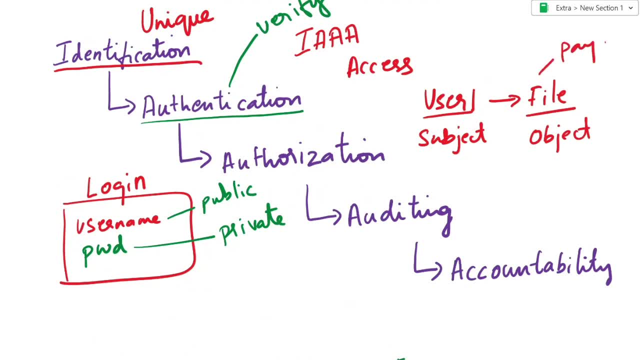 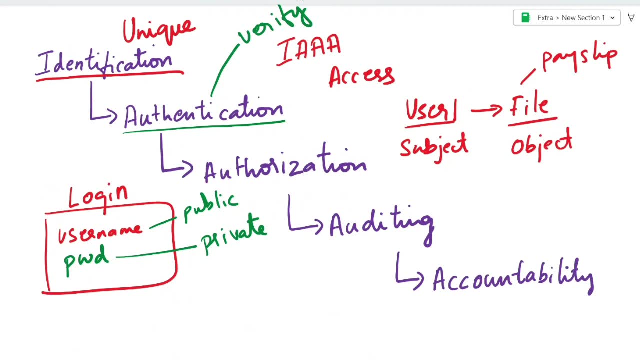 Like, for example, if the file say it is a payslip user 1, that is supposed, say Navya wants to access her payslip, I should be authorized only to look at my payslip and not the other payslips of the. 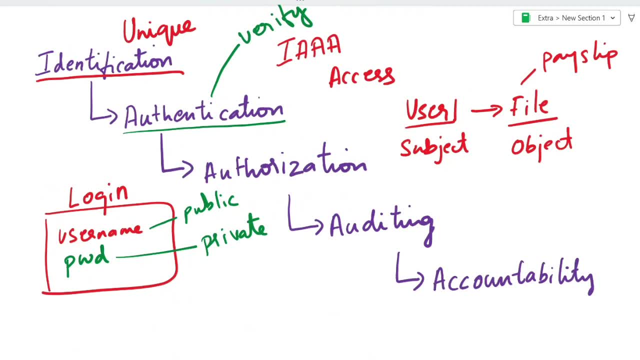 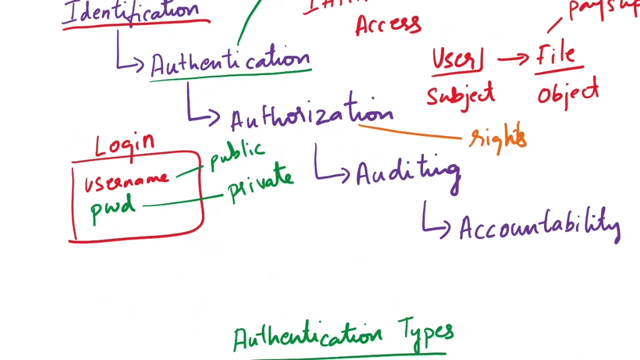 employees. right, That is authorization. Like, for example, when you board a flight, you're only supposed to take your seat. You cannot enter the cockpit because you're not a pilot. You're not authorized to be there. That is authorization. Authorization is the rights and permissions that 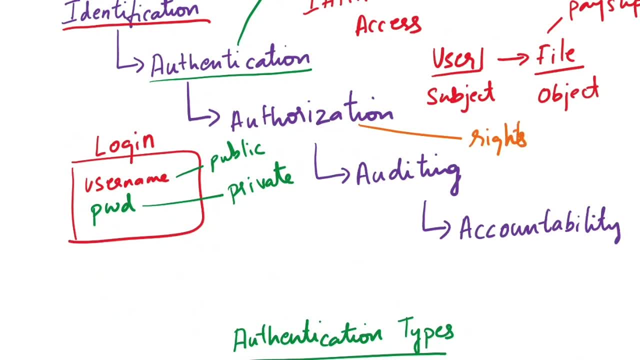 are assigned to the subject, That is, it is determining the level of access to a resource by that object, a subject, sorry So. authorization happens after authentication and then it decides which what identity can do and cannot do. Authorization is generally provided. 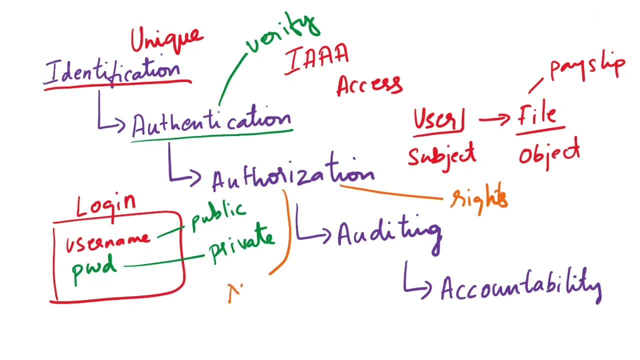 by using access control models. like you know, MAC, that is, mandatory access control, RBAC, role-based access control, rule-based access control, DAC, discretionary access control. There are many access control models that are used to provide authorization. Okay, now we have the. 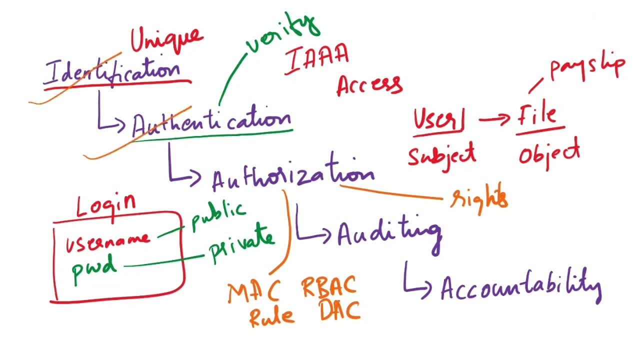 identity, and then we have verified the identity. That is authentication. And then we have also decided what the identity can do and cannot do. That is authorization. Next is auditing. Auditing is monitoring. What is it monitoring? It is monitoring the actions that are taken by the. 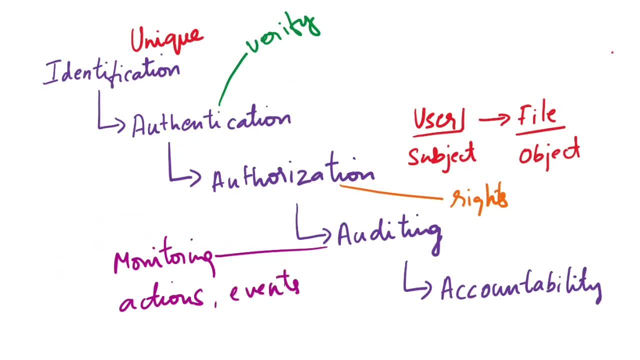 identity or the events that are related to that login right. Auditing is the programmatic means taken by the subject. It is nothing but recording the events. okay, The purpose of doing auditing is to establish accountability And all these details are recorded in a log file. okay, Auditing is not. 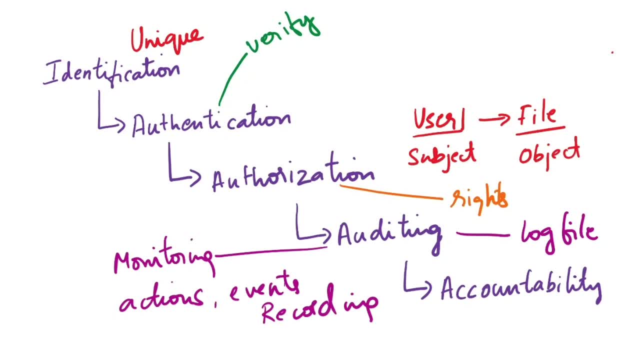 just recording the subject and objects events, but it also collects logs related to the system, Like, for example, operating systems and many of the applications and services. they have native feature of logs. So why is auditing required? It helps us to detect any malicious activities, any unauthorized 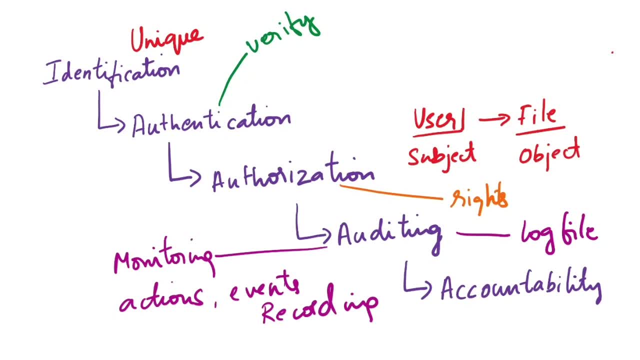 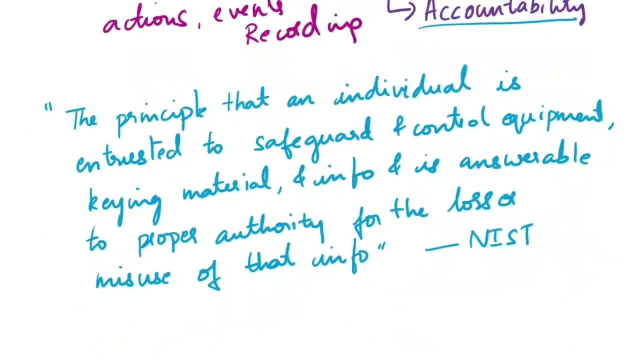 activities. It helps us to validate the compliance, the security policies of the organization. It also holds the subject accountable for their actions or activities. okay, So the next concept is accountability. According to NIST, the accountability is defined as the principle that an individual is entrusted. 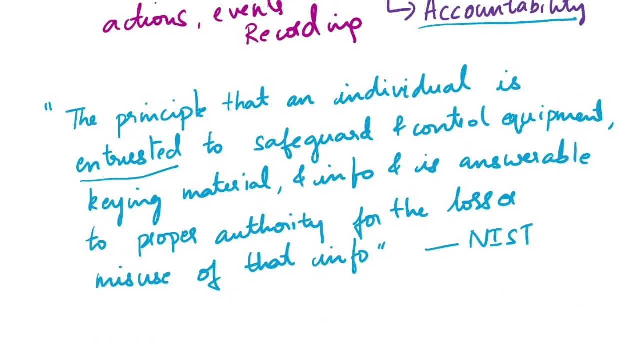 To safeguard and control equipment, keying material and information and is answerable to proper authority for the loss or misuse of that information. So to put it in simple words, right Accountability is the ability to hold an individual, that is, a subject, user process. 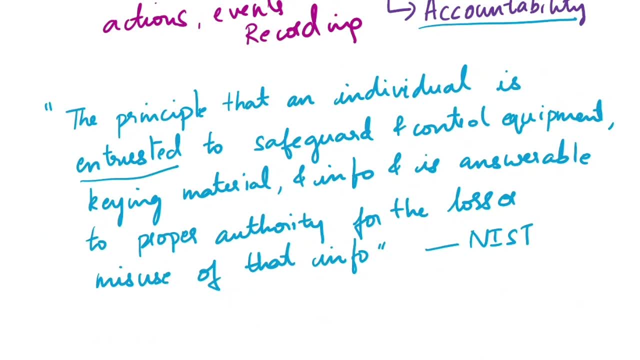 application accountable for their actions on an object, On an object. object can be a database file application system anything. Object can be a database file application system anything. And why do we require accountability? Because it ensures that every information asset is owned.